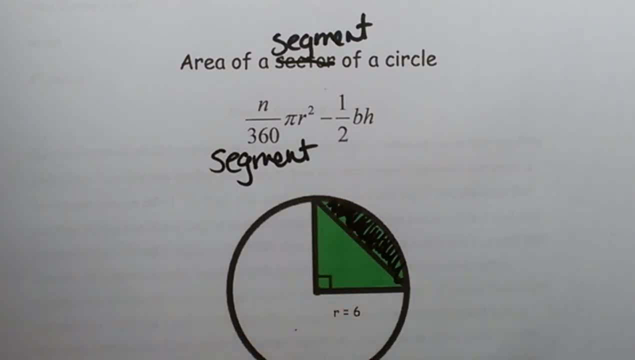 Then we are going to take and subtract out the area of this triangle. in this case we have a right triangle, so it is going to be fairly easy. So triangles you have to use different formulas for, depending on what you have, but in general 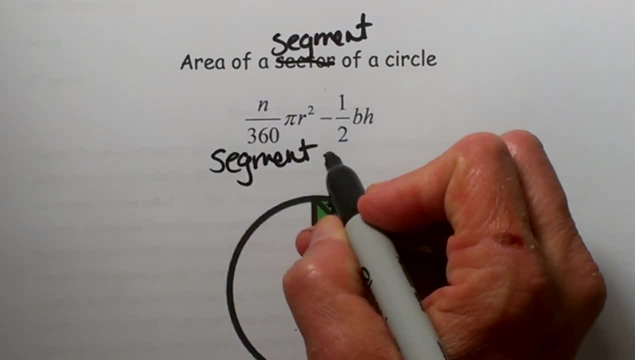 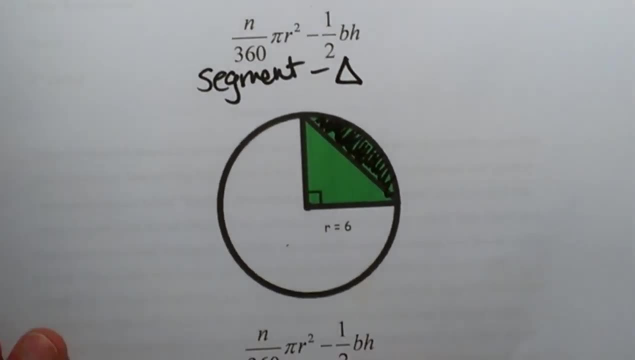 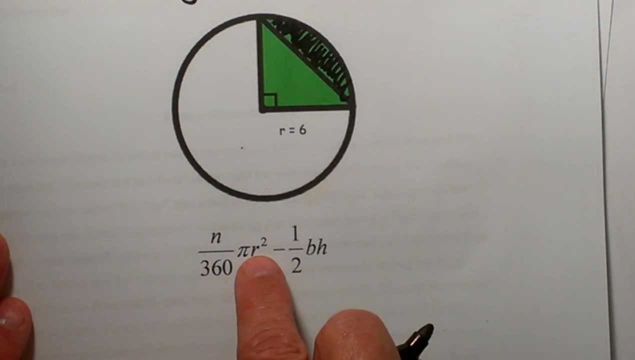 it is going to be 1 half base times height. So then we are going to take the area and subtract the area of the triangle and what is left will be this segment. So let's work through this one. So we need to know the angle measure we are dealing with is n, r, is our radius, and then 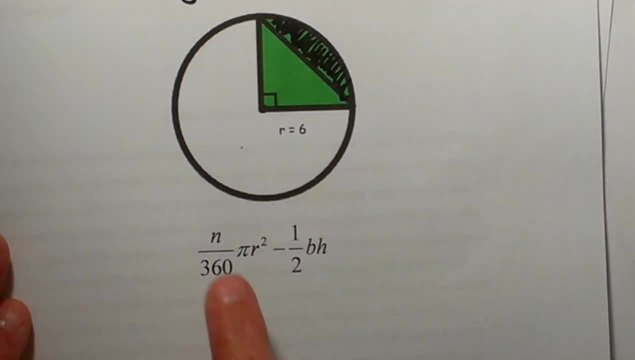 our base and height. This is inside this triangle, So let's start plugging in. Well, in this triangle, we know that our angle is 90 degrees, So that is really just 1 fourth of our circle, and the area of the circle is pi times radius. 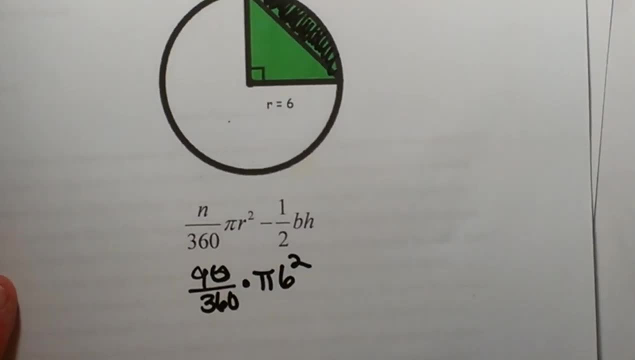 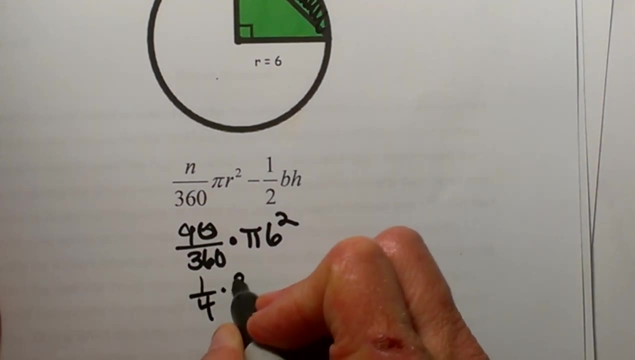 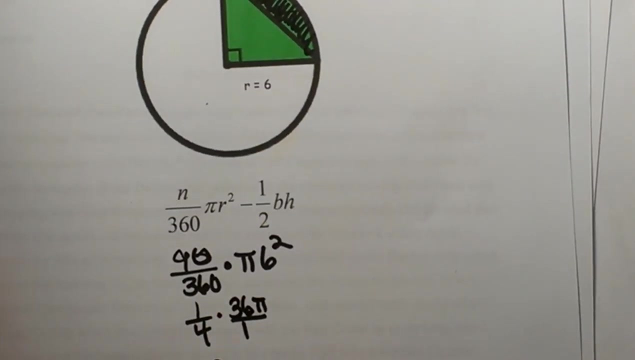 and our radius is 6, so pi times radius squared. So let's go ahead and figure out the area of this whole sector. That is 1 fourth of 36 pi, So that ends up being 9 pi. So that is the area of the sector. 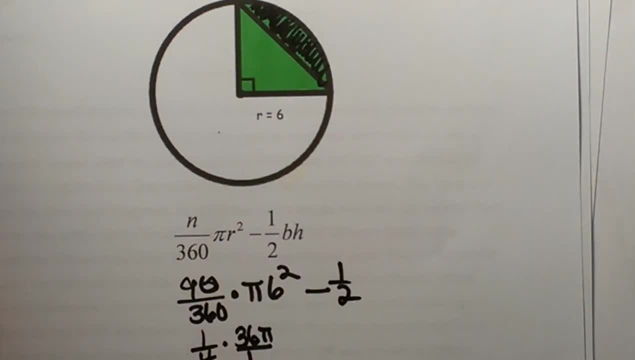 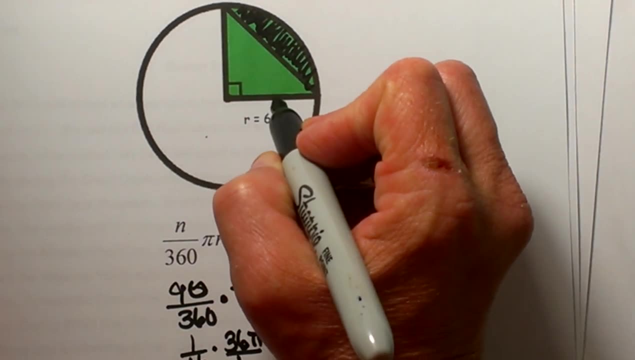 Now let's subtract off our triangle 1 half base times height. Well, the base and height on a right triangle is just the radius, So this measures 6 and this measures 6. so I am going to do 1 half of 6 times 6.. 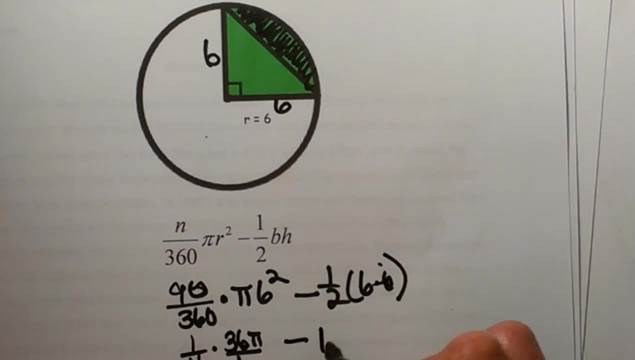 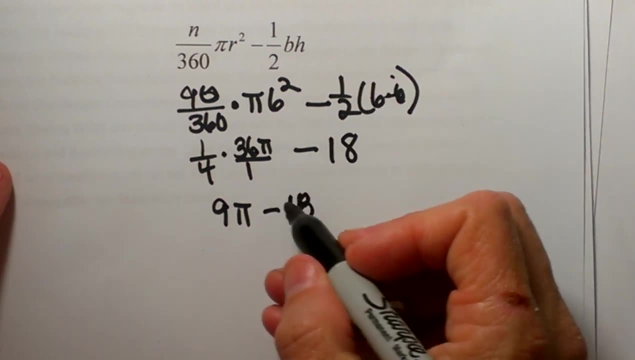 So 1, half of 6 times 6 is 36 and half of that is 18.. So that means I am just going to subtract 18.. Ok, So there is basically the area. Now that is an exact value. If they want exact, you leave it like this, or you can always go to your calculator and 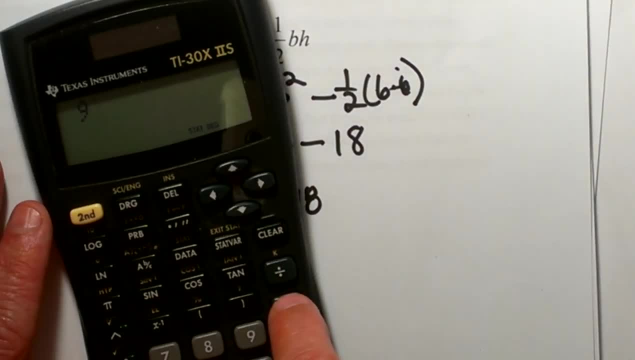 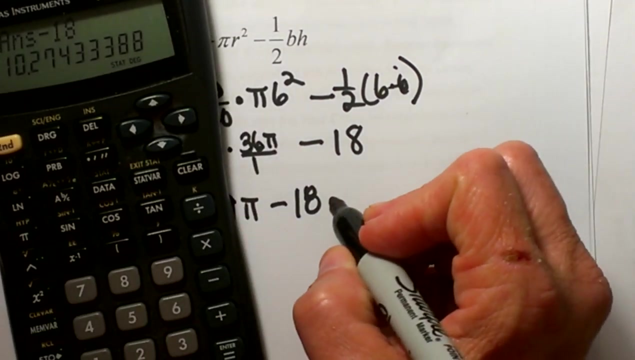 get the decimal by taking 9 times pi, and pi is right here. so I am going to click my pi button and I get 28.27, and I am going to subtract 18 from that and that gives me 10.27.. So that is an approximate value. 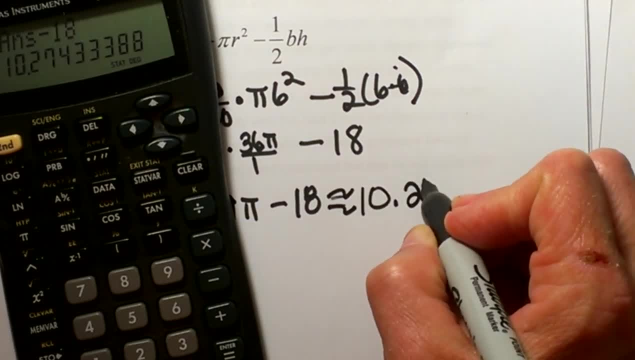 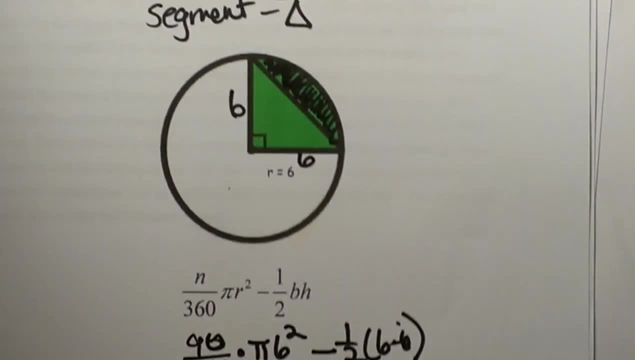 10.27.. Ok, So that is the area of the segment, or the pizza crust. Hope this video was helpful.